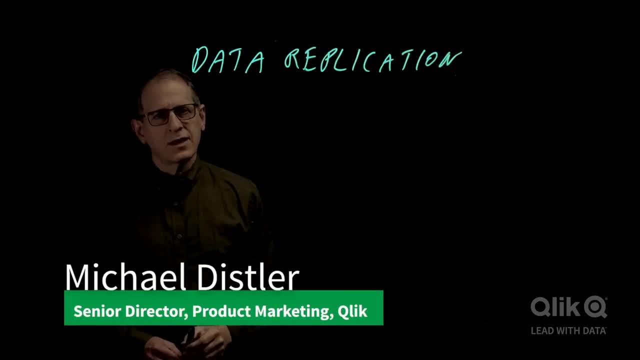 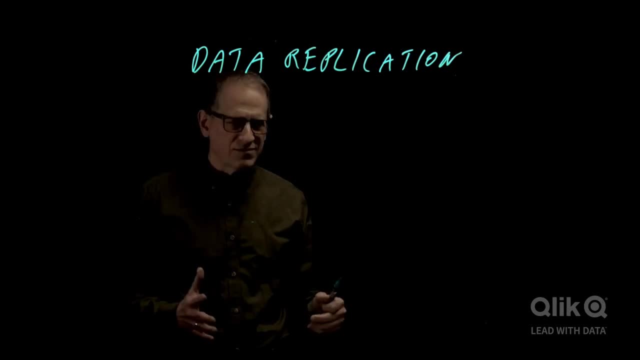 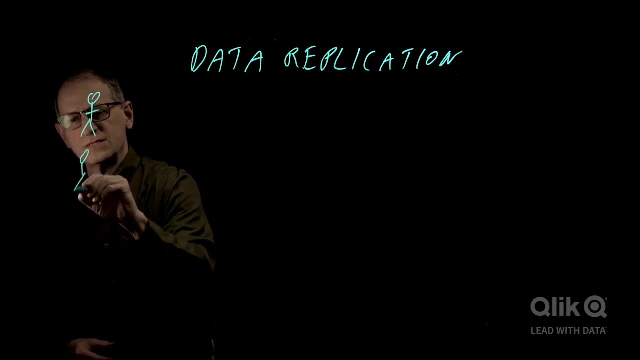 Hi everybody. this is Michael Dissler from Qlik and I want to spend a few minutes talking to you about data replication. Okay, so let's start by talking about some of the typical issues that data replication addresses. So everybody's talking about data. Everybody wants data these days. 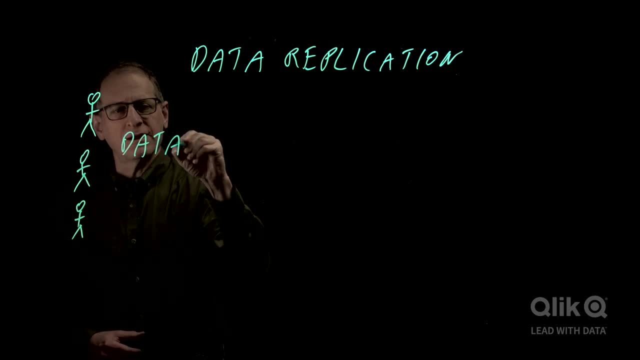 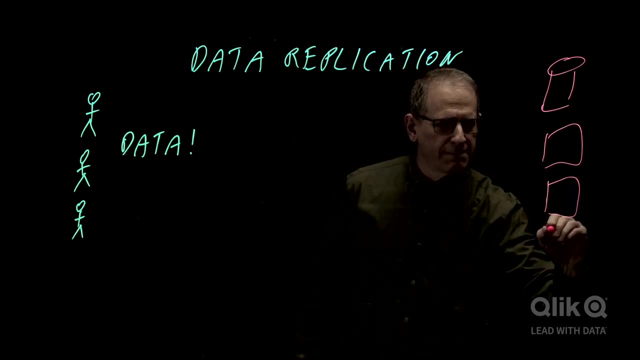 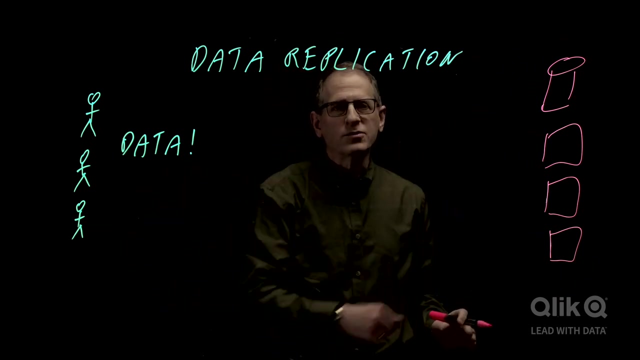 All these users over here. they want data. And then on this side you have all the different types of repositories with all the data in it, And to get data from some of these repositories, not a big deal. As many users as you want can pull data out of the repository. 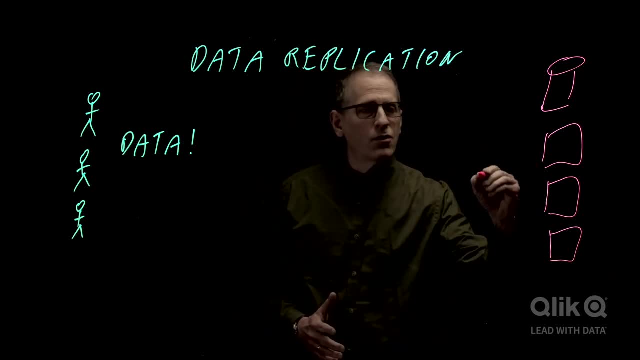 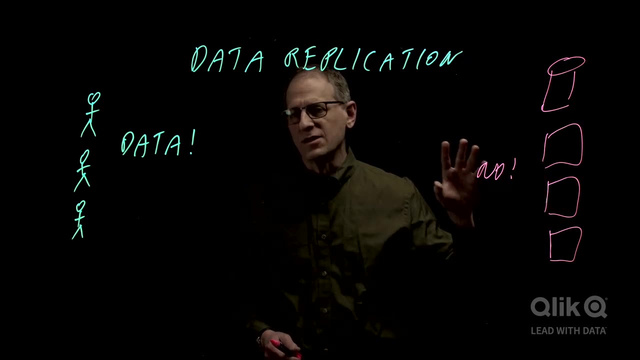 But some of these repositories, the owners of them, they might be saying no way. too many people, too many queries to my data source. It's going to really affect performance. It's really going to affect the overall performance of the system. 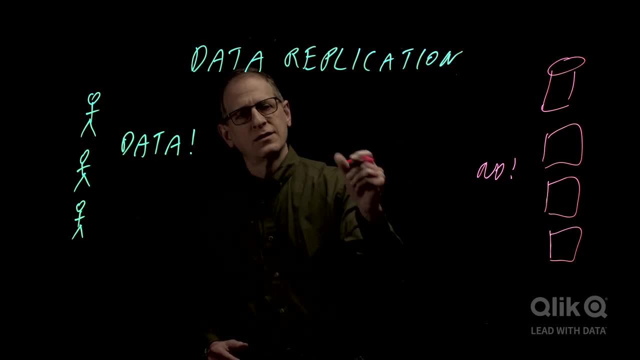 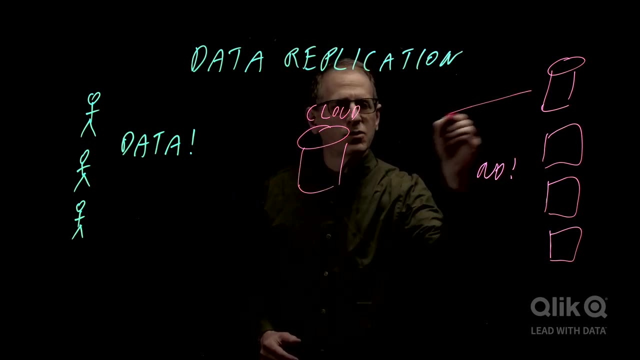 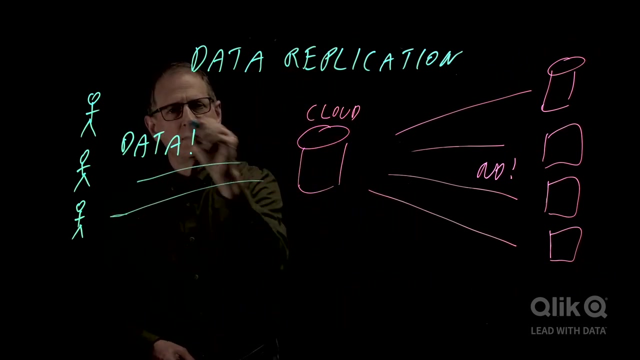 So what's needed is something in between, And typically these days it's a cloud data warehouse, And so what happens is now is you pull the data from all these different repositories into this cloud data warehouse And then these users are pulling the data from there. 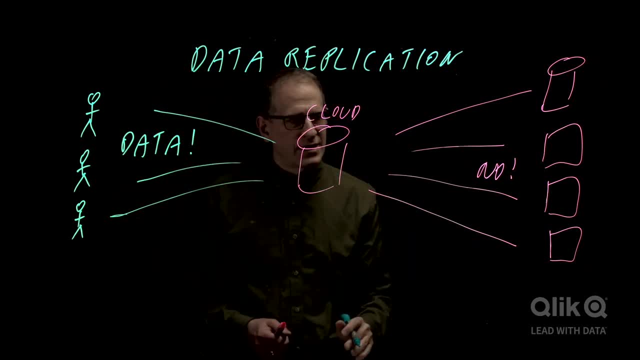 So that's incessant- is what we're talking about in data replication. Now, it can be pretty simple. If this is, for example, a relational database over here and it's a relational database in the center here, that's pretty simple to replicate. 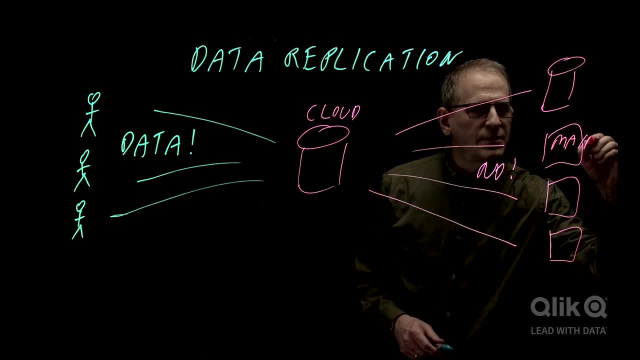 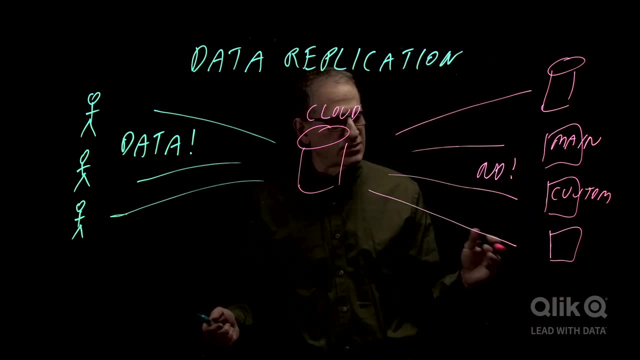 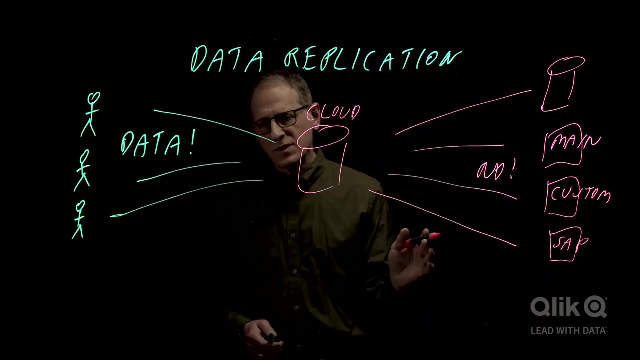 But what about? Perhaps you have a mainframe type system, Or perhaps you have some type of custom system that only your organization has ever built, Or you maybe have some complex enterprise application like SAP. Replicating that type of information is much more complicated. 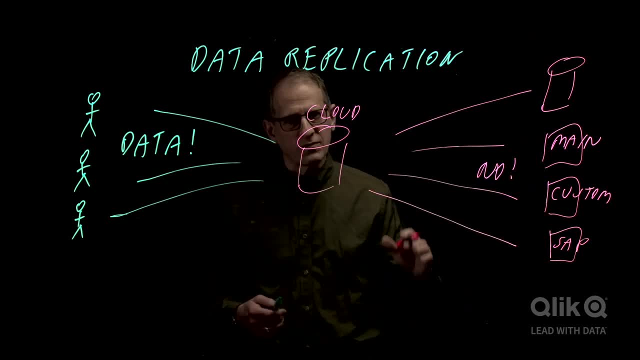 So it's important to keep in mind what you're replicating from and that you have the tools to replicate from all these different types of repositories. The other thing to keep in mind is that when you are populating this cloud data warehouse, it's really two things. 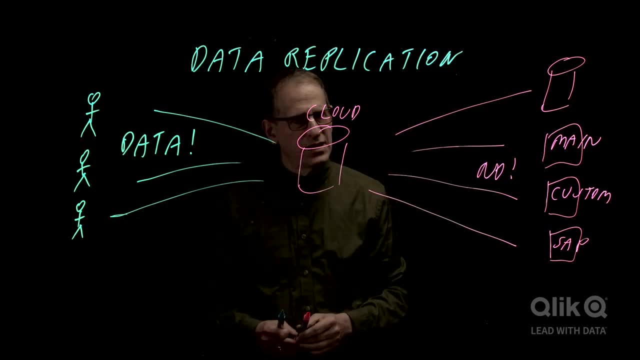 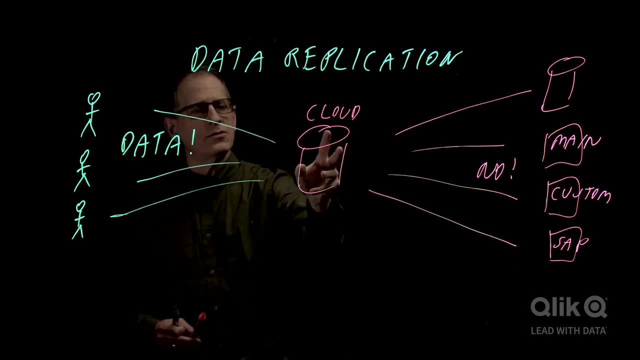 One is the initial population of that database. But then how do you keep it up to date? How do you keep all these different repositories? when a change happens over here, How do you make sure that's reflected in that cloud data warehouse as soon as possible?